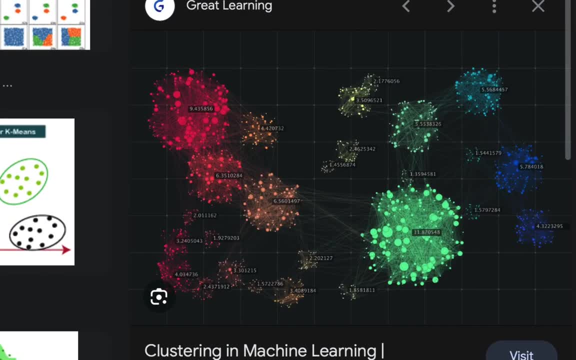 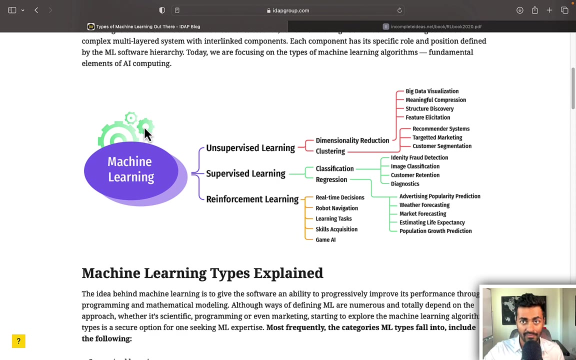 tasks and regression tasks. Then in unsupervised learning, we have data but we don't have the labels, And this is primarily used to understand patterns within data, primarily used in clustering and dimensionality reduction. And then we have reinforcement learning. Reinforcement learning is learning what to do. that is how to map. 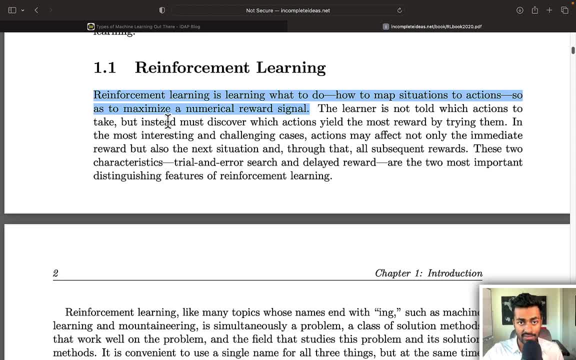 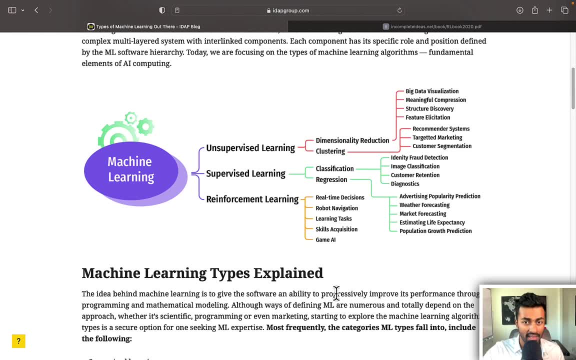 situations to actions, so as to maximize a numerical reward signal. Now, this definition is great, but it's kind of vague, And the idea now is: how exactly do I go about thinking about building a robot that knows how to navigate the world? or building some game AI? We can do so. 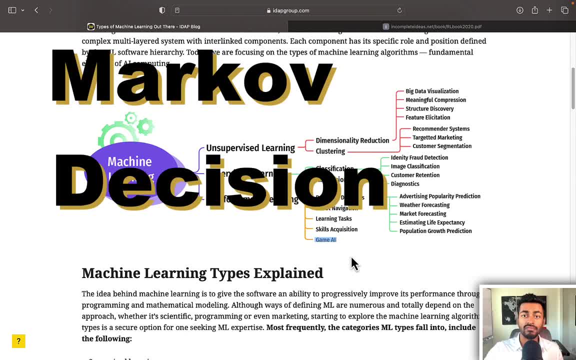 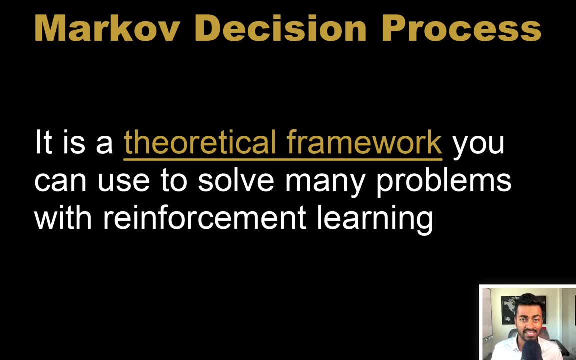 with a theoretical framework called a Markov decision process. Let's start with the simple definition. A Markov decision process is a theoretical framework that you can use to solve many problems with reinforcement learning, And here is a visual of that: MDP In a Markov 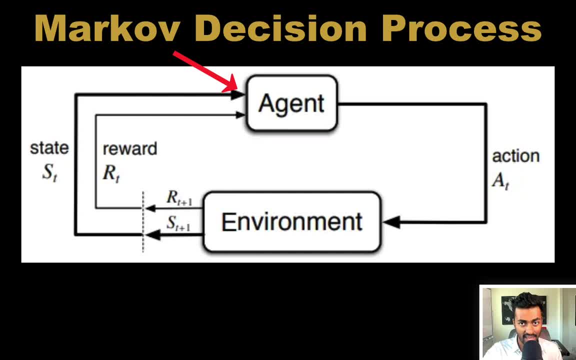 decision process. we have two main characters, that is, an agent and an environment. So the agent will perform some action in an environment and the environment in turn will emit a state and a reward And this is consumed by the agent and influences the agent's. 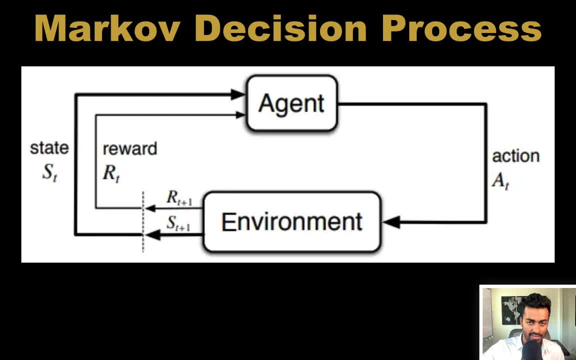 next action and so on. So this is a schematic of the Markov decision process. It is Markov, because the next state is emitted by the environment, only depends on the previous state and action. In other words, it's memoryless And past states beyond the current state don't really influence this. 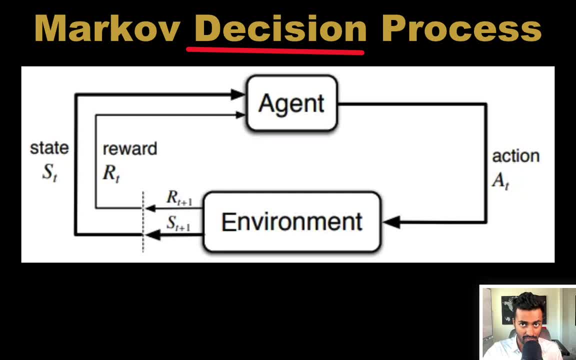 future state. Decision in Markov decision process refers to the fact that we select an action based on the current state And this leads to a state transition and the accumulation of rewards, And then we have a process in Markov decision process. Process emphasizes the interaction. 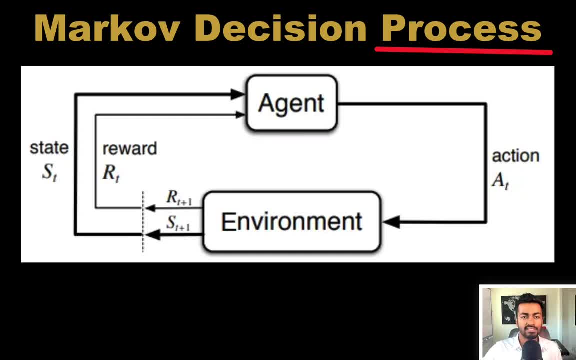 between the agent and the environment as a sequence of steps. So the agent's decision and the consequences of those decisions unfold as a process where each step is influenced by the current state and action. This setup gives more of a concrete starting point to think. 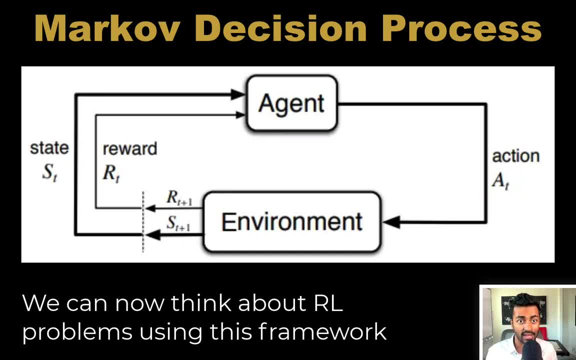 about solving problems with reinforcement learning, And so when thinking about this problem and solving it with this mindset of the MDP framework, we need to define the agent, environment, action space, the state space and the rewards. So let's do that, considering a few distinct cases. 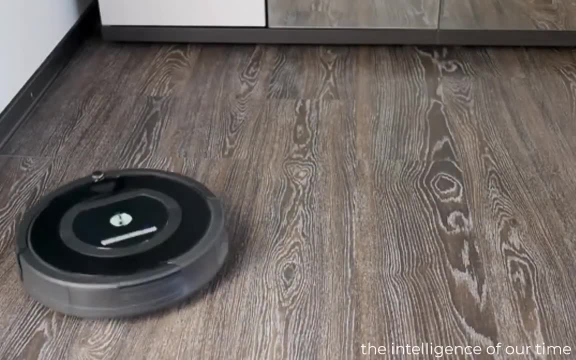 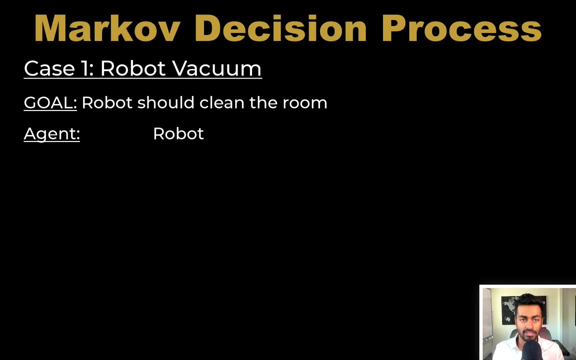 So let's say, in this first case, we want to create a robot that can clean the room, And so let's go on defining the components of the Markov decision process. So we have an agent that is the Roomba itself. 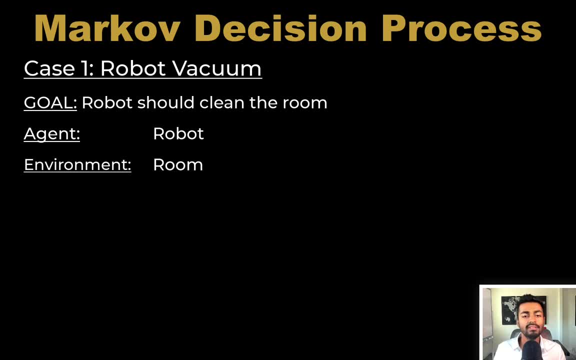 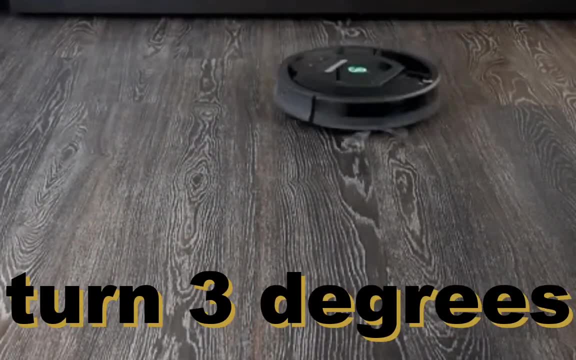 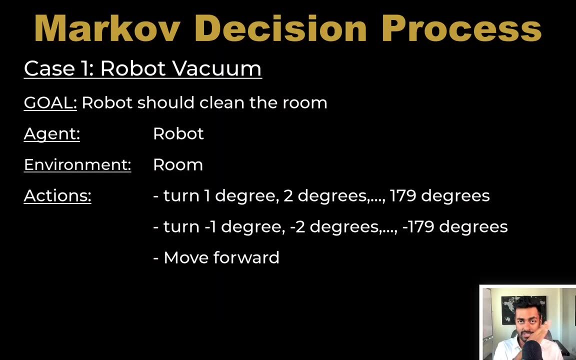 Then we have an environment, and this is the room, And the actions that the Roomba can perform are: it could be turning one degree, turning two degrees, turning three degrees, turning four degrees, until maybe like turning 179 degrees, And then it can also be in the opposite direction. 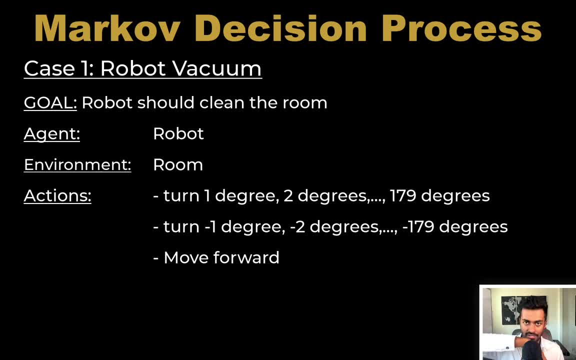 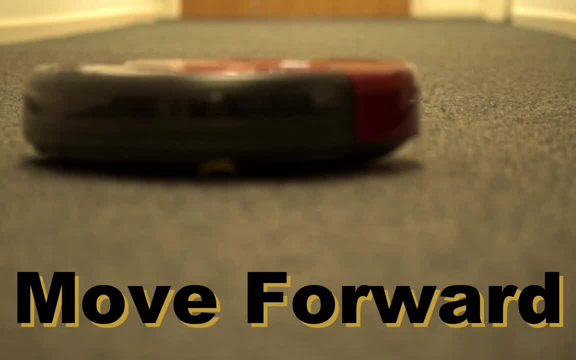 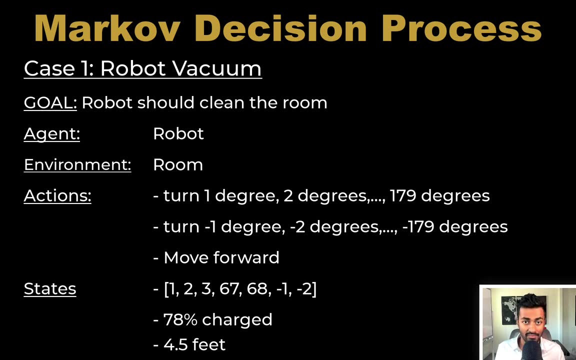 of turning negative one degree, turning negative two degrees and then up to turning negative 179 degrees, And another action could be just to move forward. Next, we want to define what is the state. So a state is a snapshot of the environment And in this case it'll be a snapshot of the room. 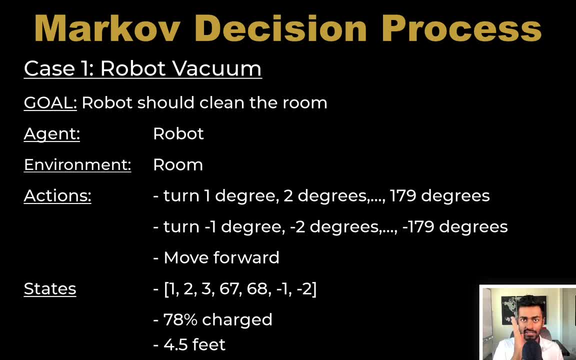 itself. So this could be the list of for every single degree. is there an obstacle within six inches? Within one degree, two degrees, three degrees: is there an obstacle within six inches? It could also be how much charge the Roomba has. 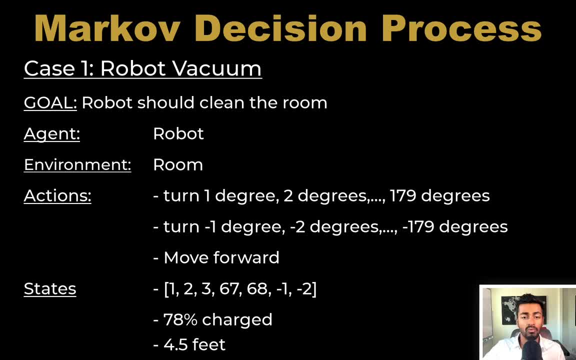 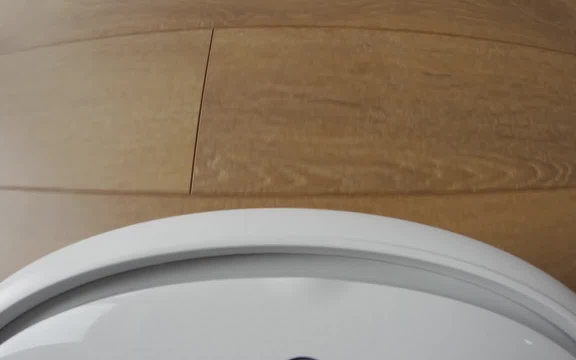 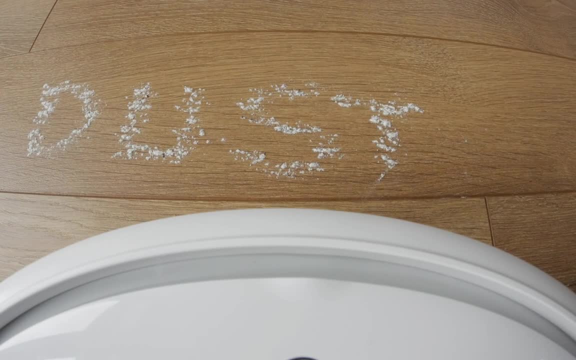 Or how far is the Roomba from the charging port, And the reward this could be the volume of dust that is collected in the container, And the idea here is that the more dust that is in the container, that means more the room has been cleaned And it goes in tandem to achieve the goal. 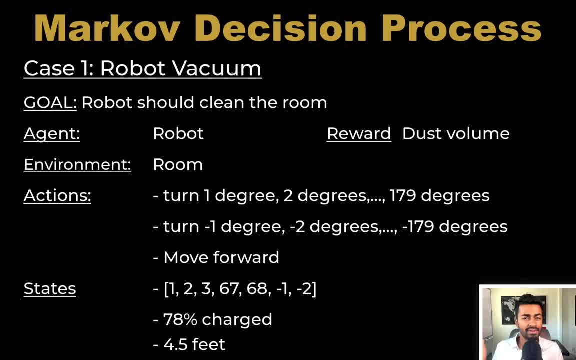 that we set out for this Roomba, And now that we've defined all of these components, it is a matter of just now collecting data and coding things out from here. Now. it's important to note here that we don't really need to think in the realm of AI. 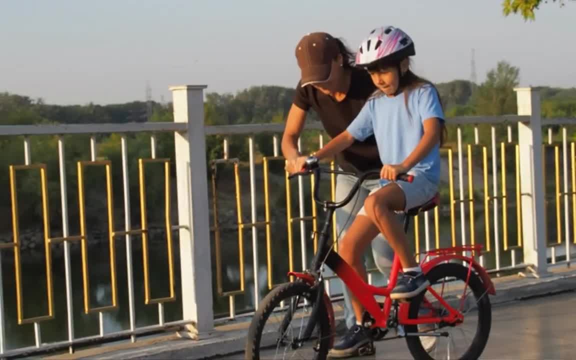 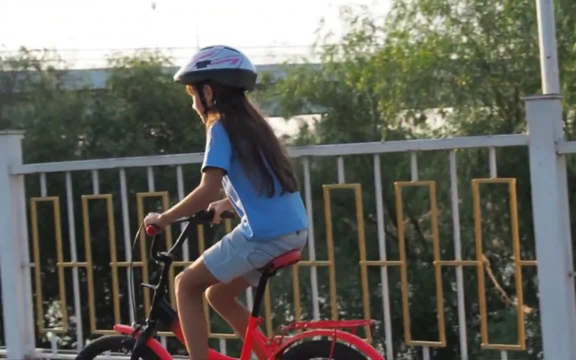 The Markov decision process can go much beyond this. For example, consider a case, too, where a human is riding a bike and the goal here is to learn how to ride a bike. The agent is the human, The environment is the bike which is on a road. The actions could be. 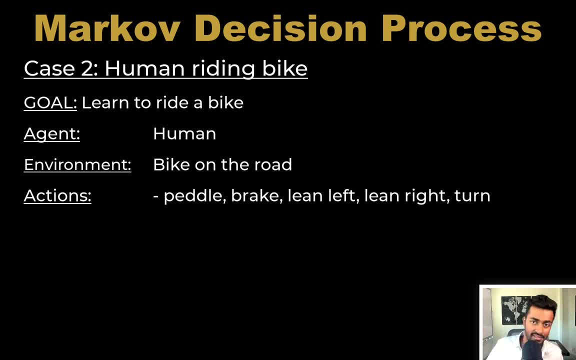 to pedal, to brake, lean left, lean right, turn left or turn right or continue straight. Now the state is a snapshot of the human on the bike on the road. Is there an obstacle 12 feet forward? Is there an obstacle immediately to the left and immediately to the right? 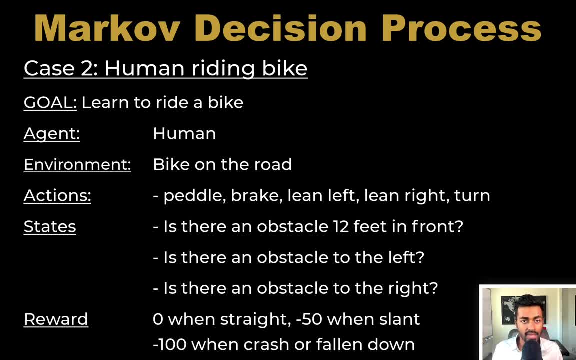 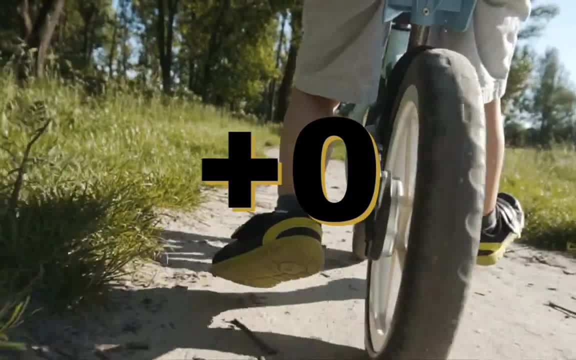 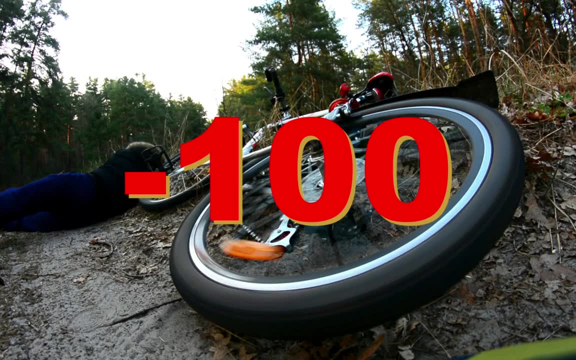 What's the direction of our destination? Next Reward: this could be 0 for every time step that the bike is straight up, a negative 50 reward if the bike slants a lot, or a negative 100 reward if we crash or fall down. 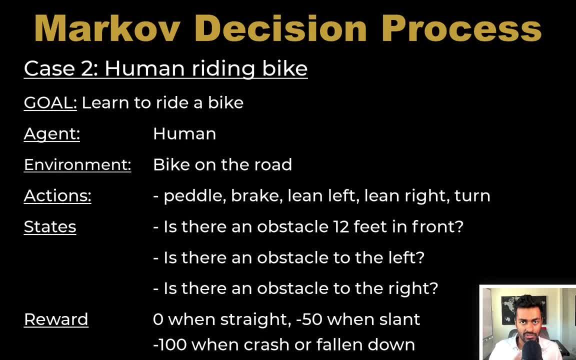 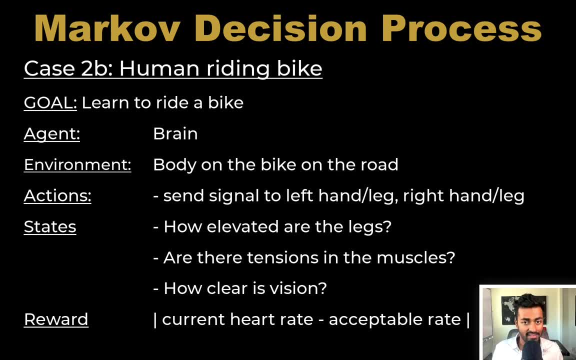 And all of this will incentivize our agent to well be upwards so that it can maximize the reward. Now, another important thing to note here is that this is just one way to define a solution to how to ride a bike. It's not the be all, end all. 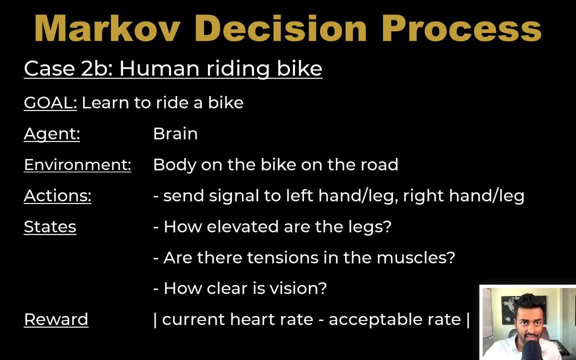 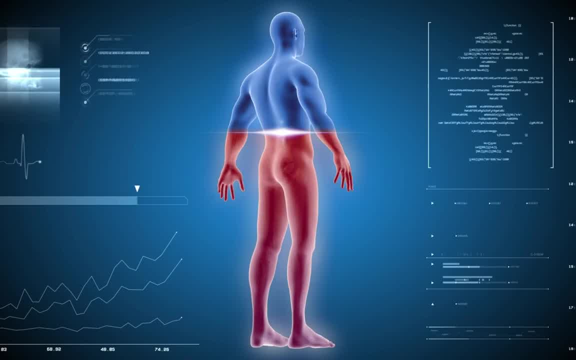 And an extreme example would have framed it kind of like this, where the agent could be the brain and the environment is the body which is on the bike. The actions are: send signal to the left hand, send signal to the right hand, send signal. 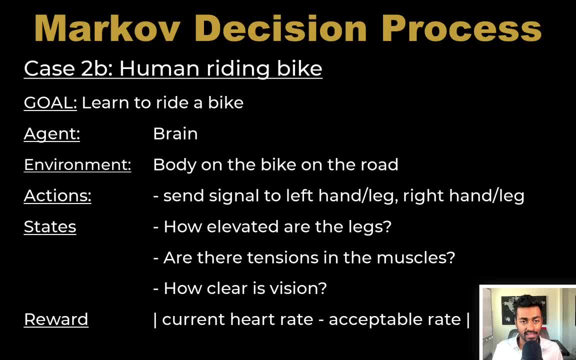 to the left leg, send signal to the right leg And the state, which is the snapshot of the body, could be: how elevated are the legs and the hands? Are there any tensions that exist in the muscles? How clear is our vision? 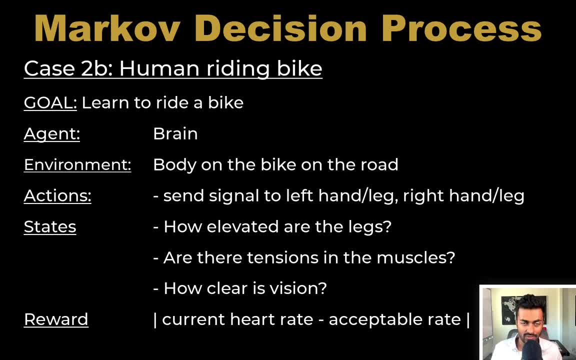 And the reward would be: what is the absolute difference between the current heart rate and the acceptable heart rate for riding a bike? So clearly, it's very fluid. Now let's talk about how we define what an agent and environment is, even for the